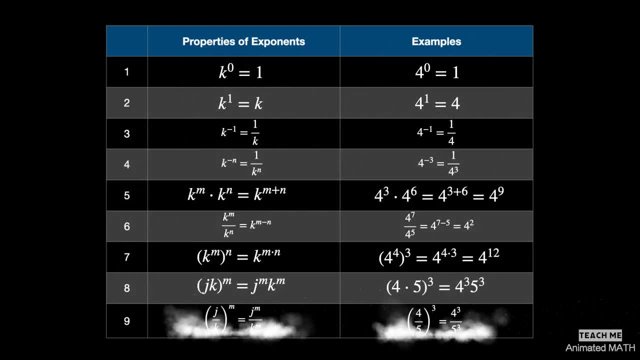 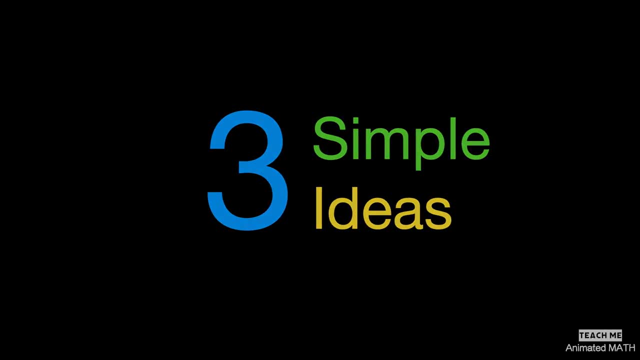 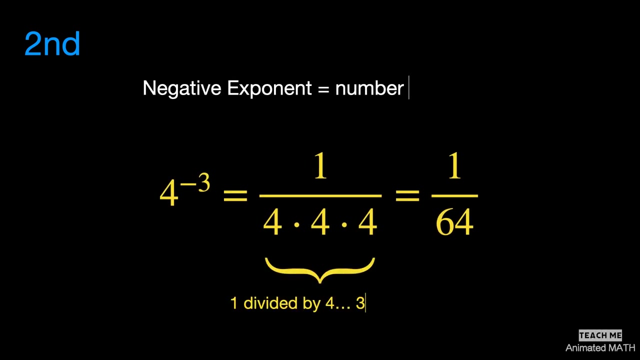 The properties of exponents might seem a lot at first glance, but really they can be broken down into just three simple ideas. First, the exponent says: how many times you have to multiply a number by itself? Second, the opposite of multiplication is division, which is why a negative exponent says: 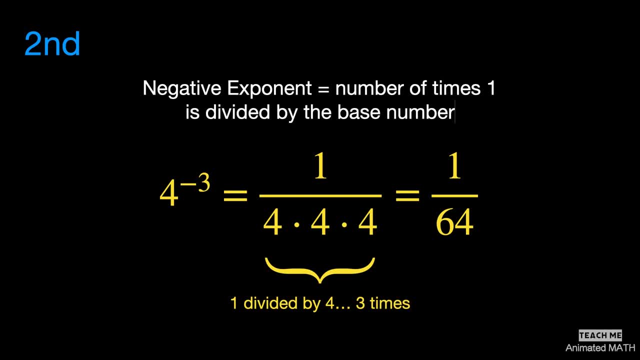 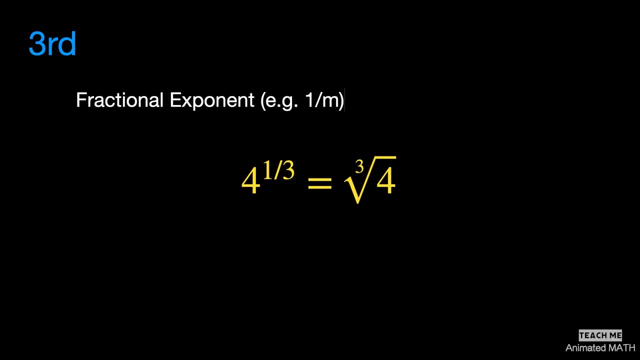 how many times you have to divide one by the base number? Third, a fractional exponent like 1 over m means to take the mth root of a number. For example, 4 raised to the 1 3rd power is equal to the cube root of 4.. 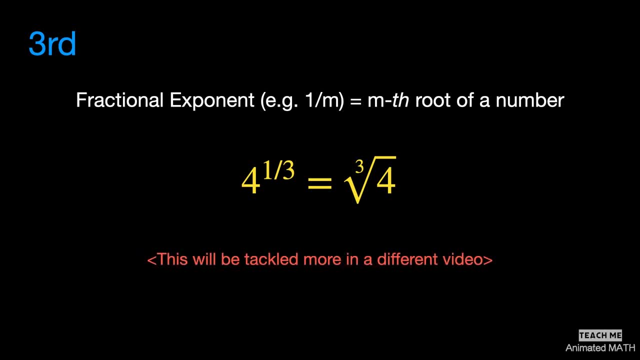 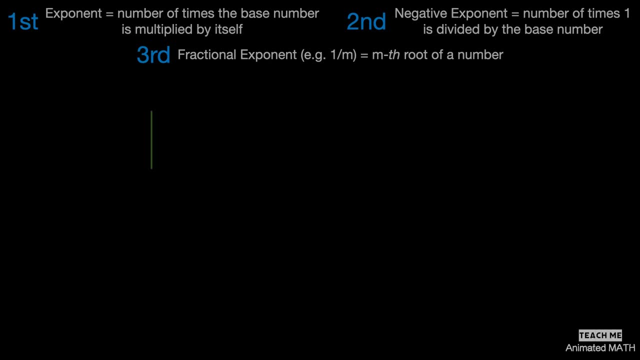 This will be tackled more in a different video. Now that you've been briefed, it'll be much faster and easier for you to understand the properties of exponents in detail. Let's start with the first three properties of exponents. Any number raised to 0. 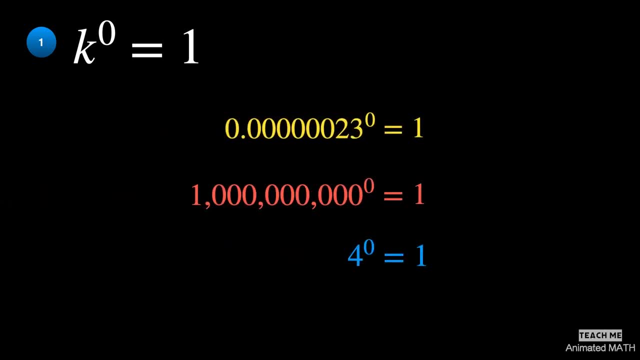 power is equal to 1.. It doesn't matter if the base is very small or if it is a million. Raising it to the 0th power will still result in 1.. Raising the base number to the 1st power is just. 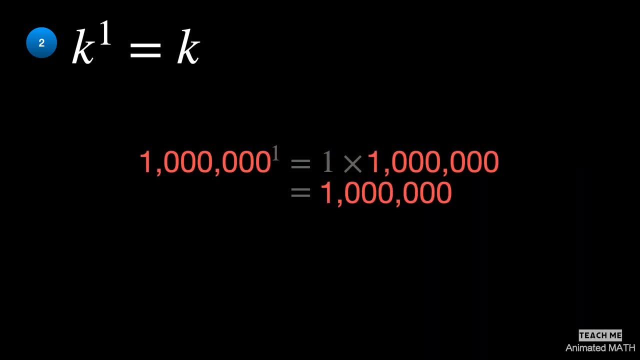 like multiplying 1 with a number. Raising the base number to the negative 1st power is just like dividing 1 with a number. In fact, you'll realize that these three properties are just part of the natural sequence of exponents. 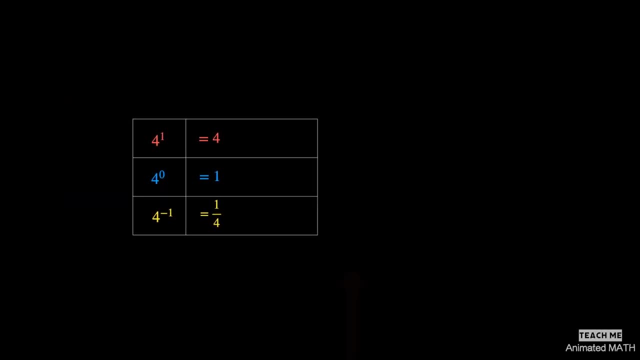 Take a look at our example of the powers of 4.. As you move up, each number is 4 times larger than the previous one, And as you move down, each number is 4 times smaller. The fourth property, A negative exponent, means that you'll have to do division. Given k to the negative n. 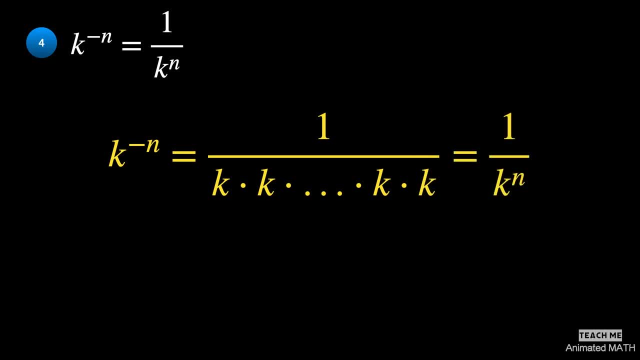 how many times do you have to divide 1 by k? The answer is n times. Here is an example: k to the negative 4 is equal to 1 divided by k, k, k, k or 1 over k to the fourth, Let's multiply the k with the negative 1.. 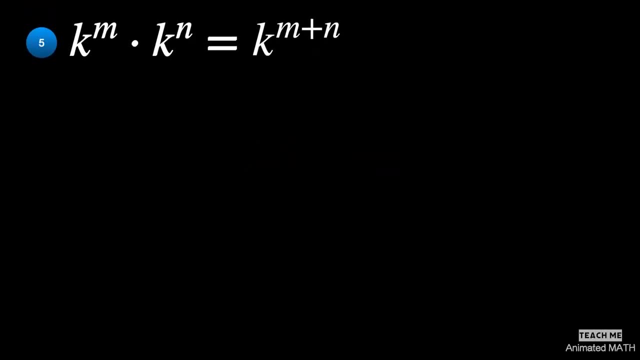 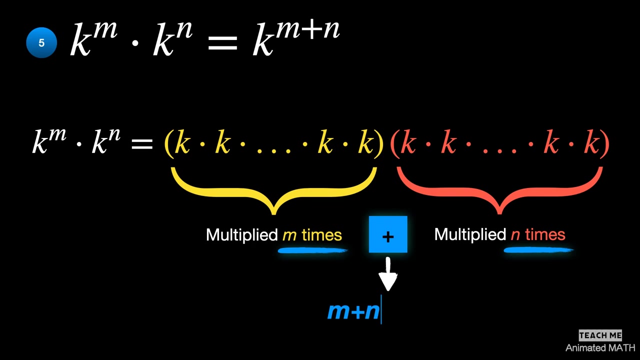 The fifth property. So given k to the m times, k to the n. How many times do you have to multiply k by itself? First multiply m times, Then by another n times. This will give you a grand total of m plus n times. 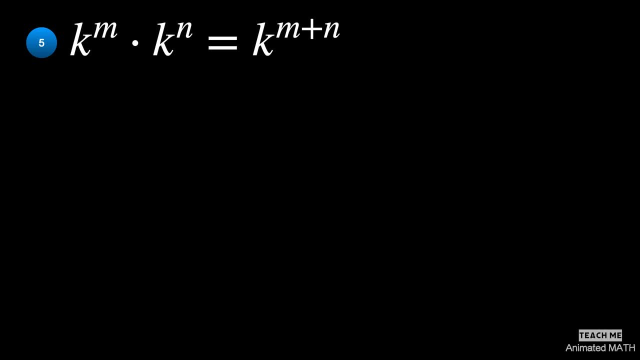 Here is an example of the experiment. For example, k to the 4 times k to the 5 is equal to multiplying k 9 times, or k to the 9th power. Using the fifth property you can write it as k raised to the power of 4 plus 5, or k to the 9th power. 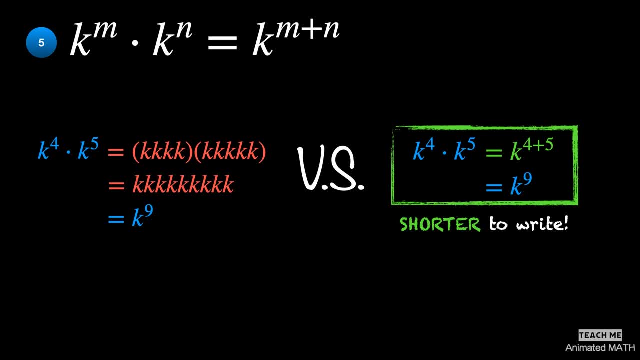 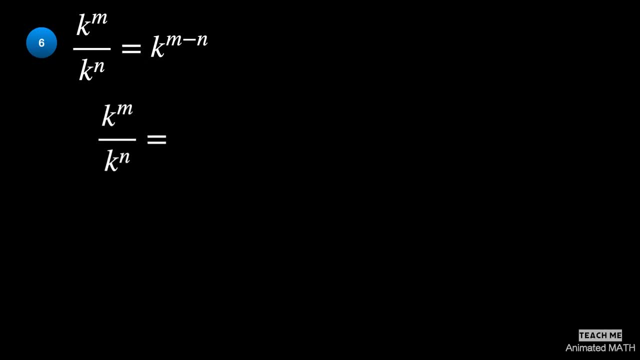 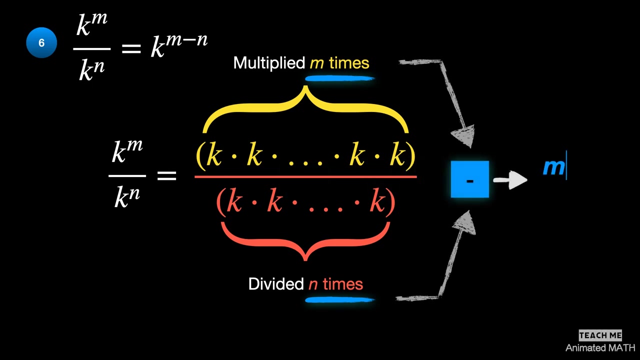 Much simpler right. The sixth property, Similar to the last example: how many times do you have to multiply k by itself? First multiply m times, Then decrease by n times because you're doing division. This will give you a grand total of m minus n times. 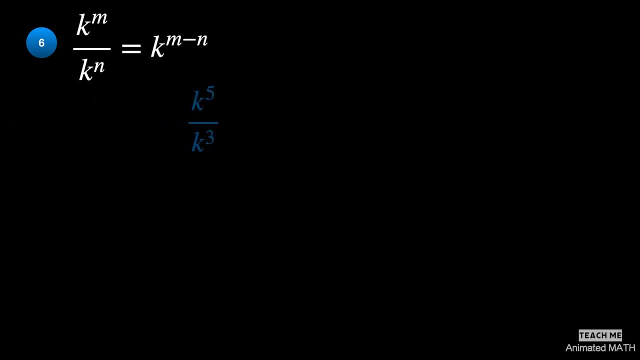 Here is an example: k to the 5 divided by k to the 3 is equal to multiplying k 5 times and dividing it by k 3 times, or k squared. Using the sixth property, you can write it as k raised to the power of 5 minus 3 or k squared. 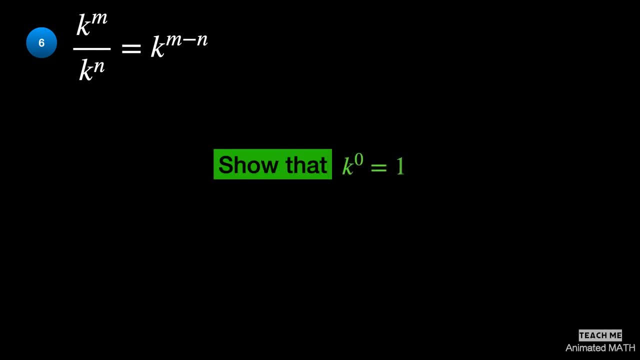 This property can also show you why k to the 0th power is equal to 1.. For example, k cubed over k cubed, using the expansion method on the left and the sixth property on the right, The seventh property: How many times do you have to multiply k by itself?